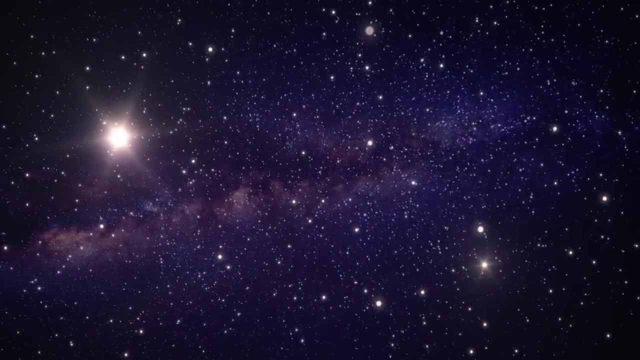 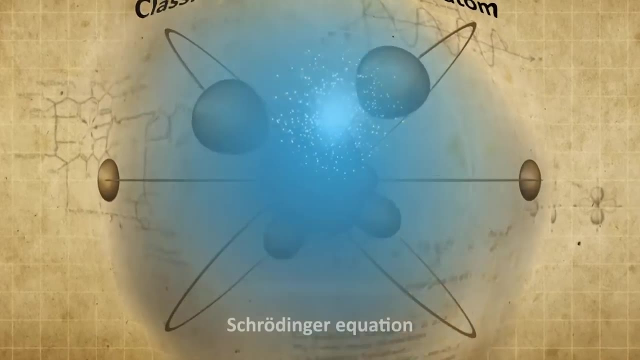 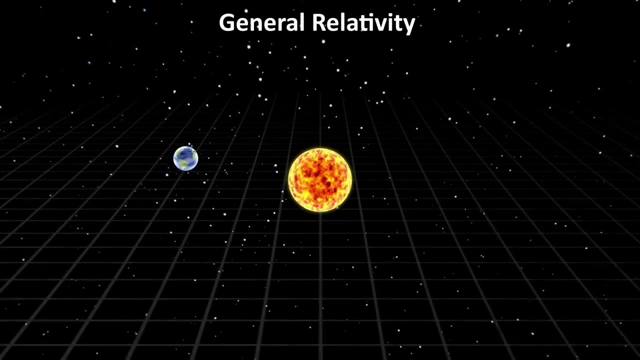 and predicted through observations and equations. In the early twentieth century, this view of a mechanical, deterministic and predictable universe was shattered with the advent of relativity and quantum mechanics. Time was no longer set in stone and the precise location of particles was no longer known, But the universe was gradually becoming more and more complex. 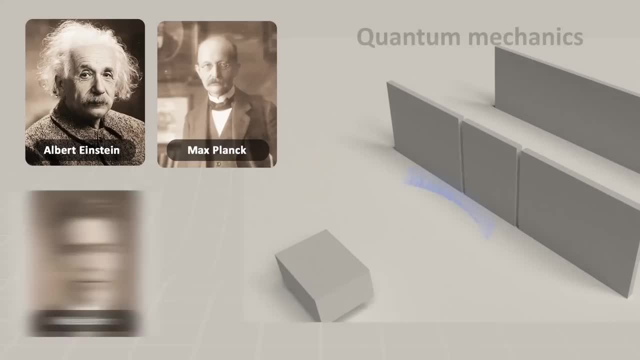 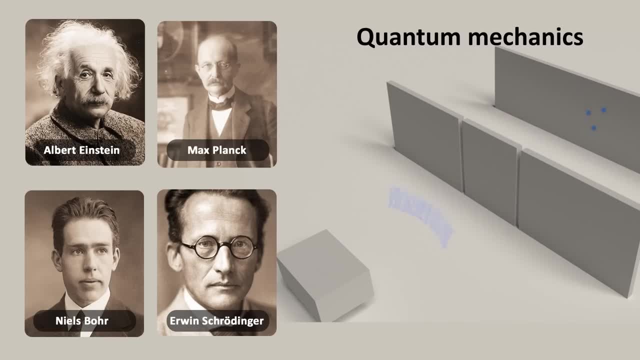 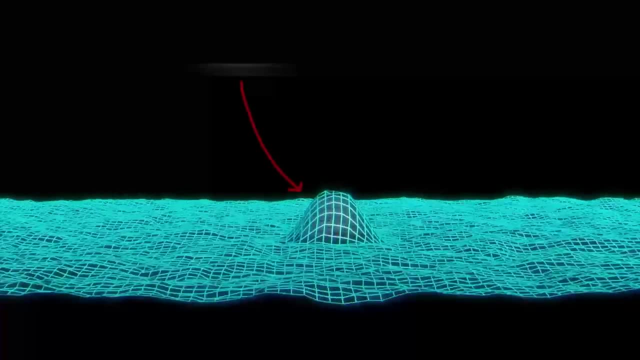 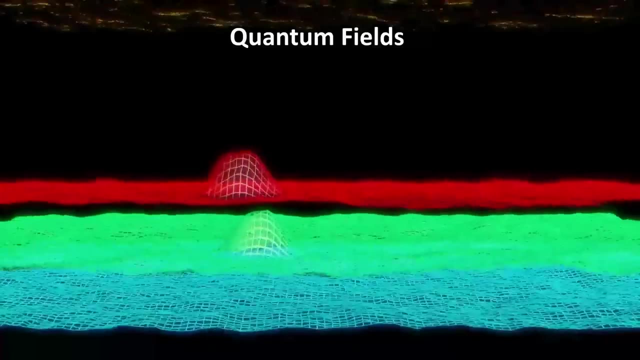 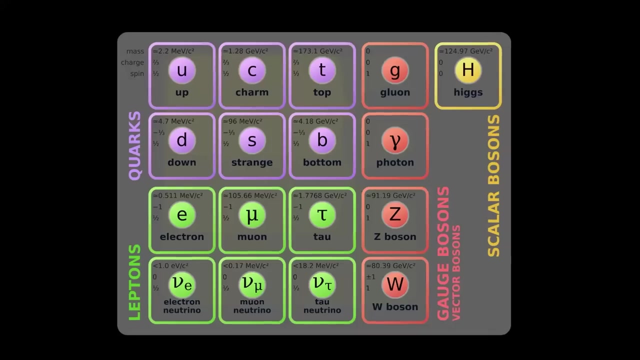 This might seem like the end of the story, but there has been one additional, more recent, paradigm shifting development in physics that perhaps did not receive as much fanfare, but it is undoubtedly equally profound, And that is how quantum mechanics was supplemented and made more complete by quantum field theory, or QFT. It is the basis of the best theory. 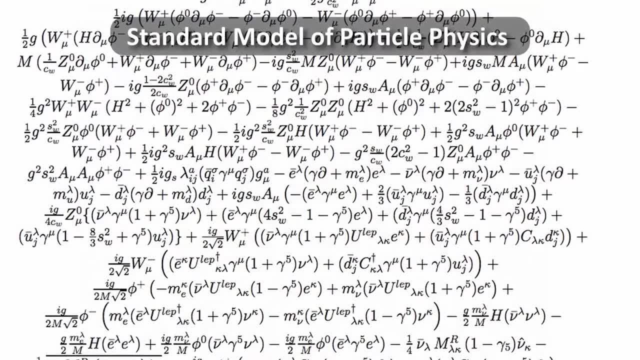 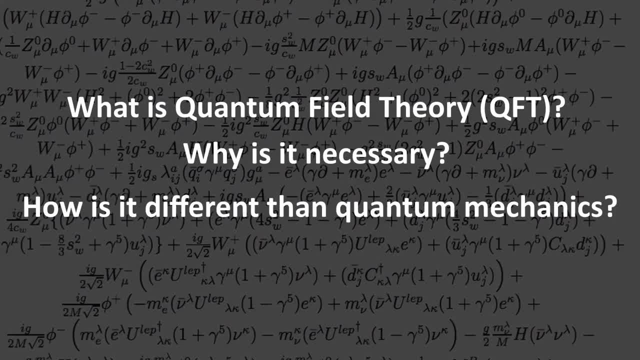 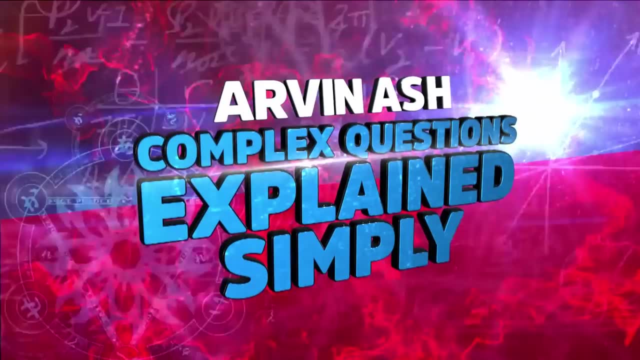 we have in physics today to explain nearly everything called the standard model of particle physics. What is quantum field theory? Why is it necessary? How is it different than quantum mechanics That's coming up right now? Classical mechanics has been and continues. 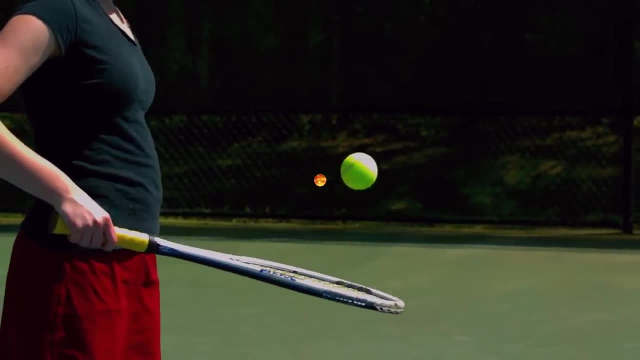 to be a fundamental phenomenon and it has been and will continue to be a fundamental phenomenon and will continue to be a fundamental phenomenon and will continue to be a fundamental use to explain many phenomena that we can observe. Consider a planet orbiting a star. 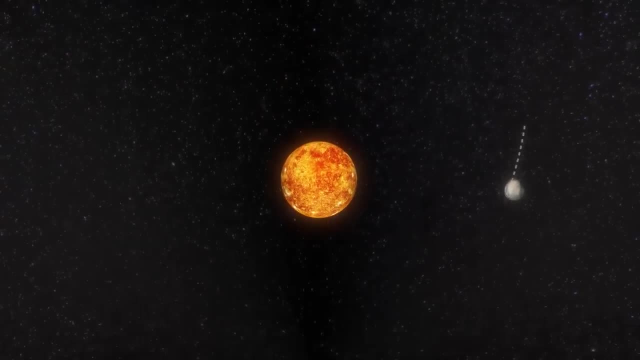 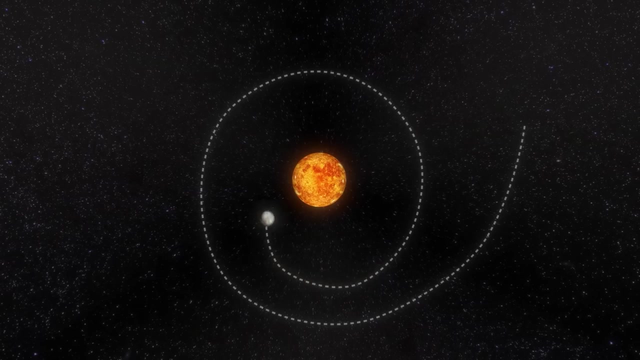 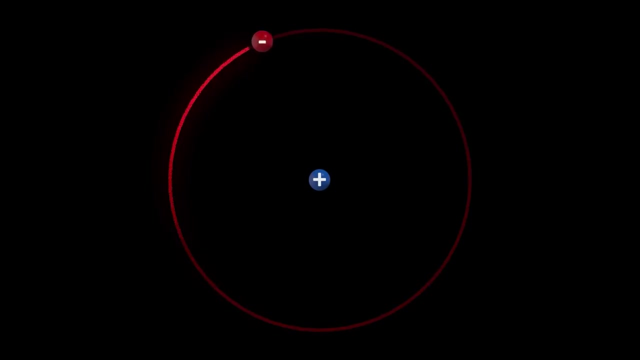 We can use Newton's laws to model it fairly accurately. If the planet were to somehow lose its kinetic energy or slow down, it would spiral into the star and collide. Consider something conceptually similar: an electron orbiting the proton of a hydrogen atom In. 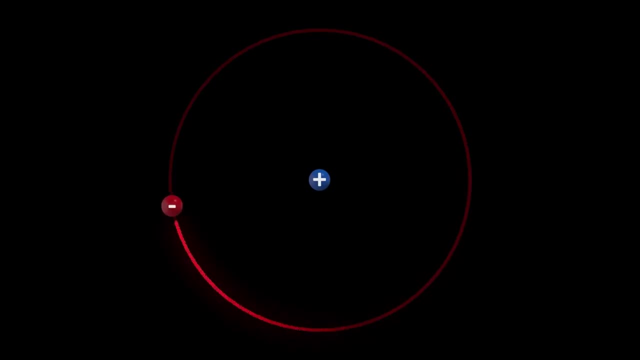 this case, we could again try to use Newton's laws to model it. instead of the attractive force of gravity for the star and planet, the two objects' electrical charges keep it bound together. This is where classical mechanics fails, because, as we know from Maxwell's laws. an accelerating charge creates electromagnetic radiation, and the constantly changing direction of the electron creates an acceleration. This means the electron would constantly give up photons, losing energy in the process. It would thus spiral towards the nucleus and collide, But we know that no such thing actually. 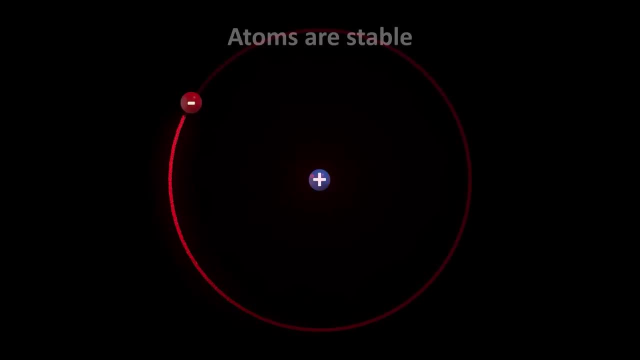 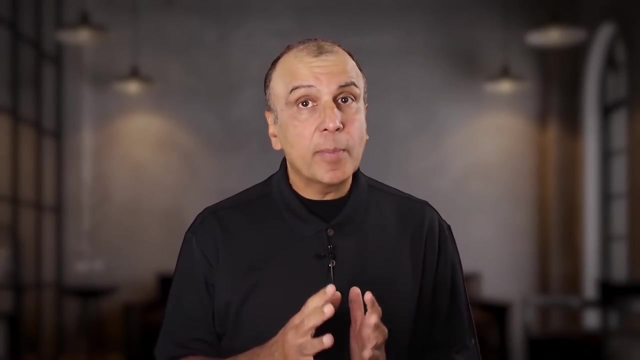 has to happen. What happens in reality? Atoms are stable. An electron does not crash into the nucleus. Why? Because we were using the wrong tool to describe the model of an atom: Classical mechanics. We have to use a new tool: Quantum mechanics. Niels Bohr proposed that the electron maintains a stable orbit because its energy is quantized. It can only be in an orbit that is an integer multiple of a minimal quanta, and its lowest energy state is an integer multiple of a minimal quanta. 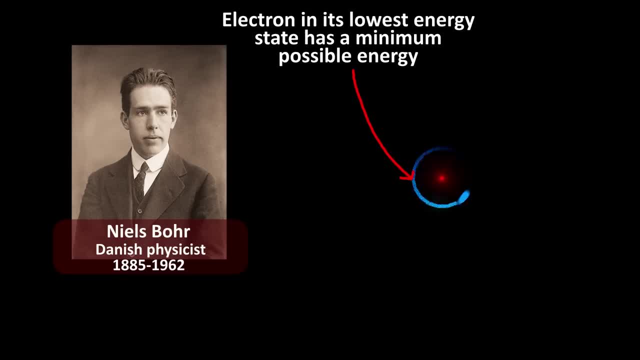 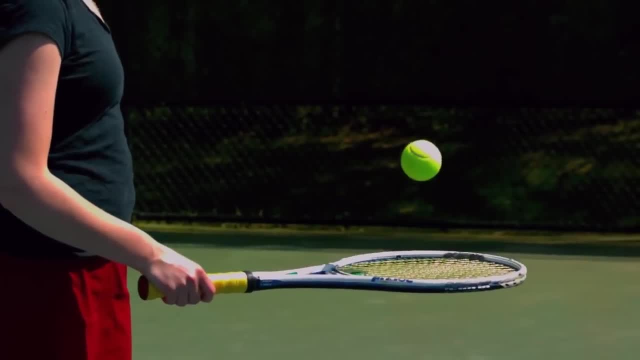 The minimum quantum state is the lowest orbit the electron can have. It cannot be lower. This minimal quanta, by the way, is proportional to the Planck's constant. In Newtonian physics we think of objects as discrete particles having very specific and measurable properties. 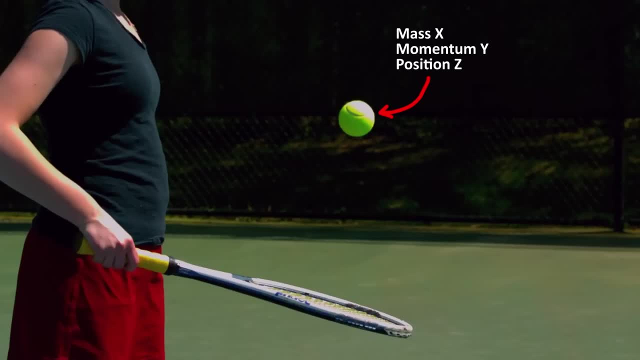 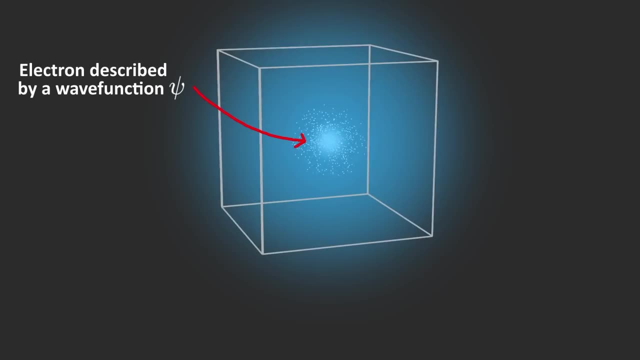 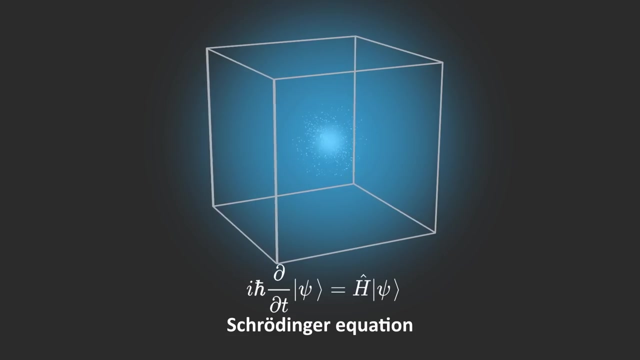 such as mass x, momentum y and position z. In quantum mechanics, our objects are wave functions described by some completely different mathematics. This is shown by the Schrodinger equation, Which is perhaps the most important equation in quantum mechanics. Here, the location of 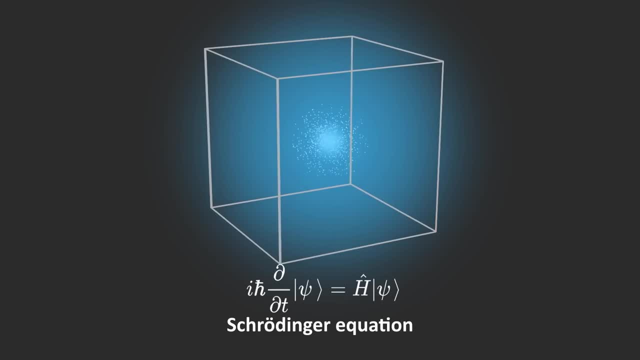 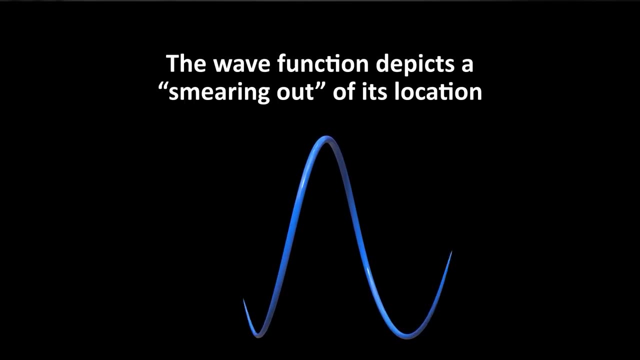 a particle is unknown until the moment of measurement. We cannot know where it is beforehand. We can only know the probability of finding it at any specific location Prior to measurement. the wave function depicts a kind of smearing out of its location. Thus in the quantum 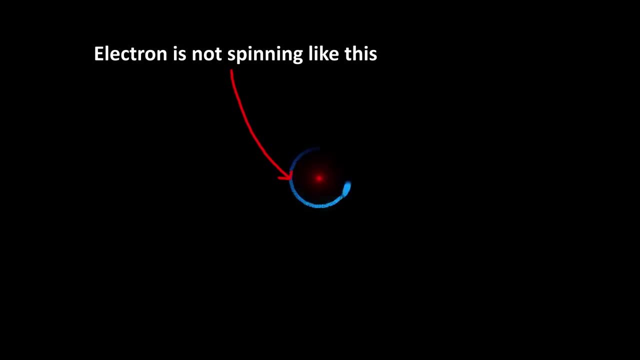 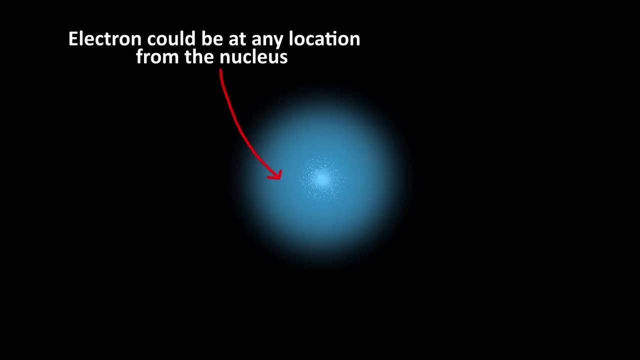 mechanical model of the hydrogen atom, the electron is not spinning around the nucleus like a planet around a star. In the quantum mechanical model of the hydrogen atom, the electron is not spinning around the nucleus like a planet around a star. It is in some unknown location, at some unknown distance from the nucleus. All we know is: 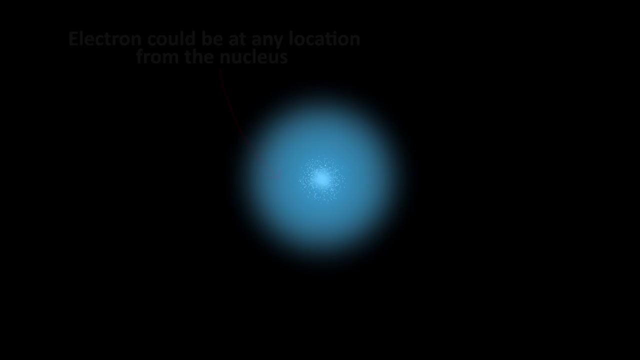 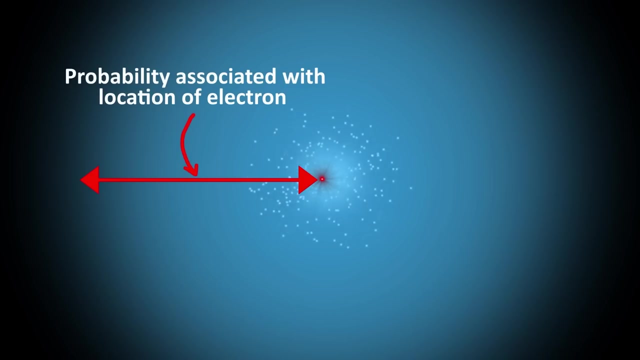 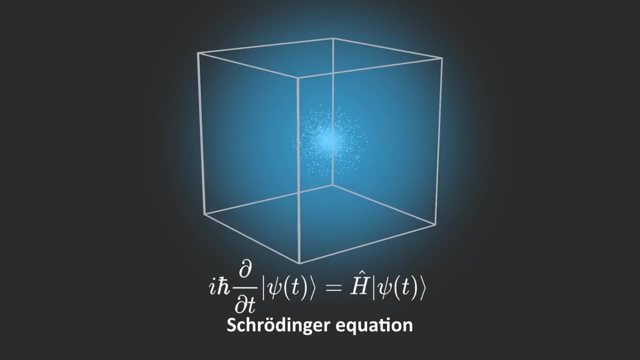 that the chance of finding the electron at any specific location or distance from the nucleus has a probability associated with it, And we can't determine the location in advance of measuring it. So the better model of the atom is like a cloud around a fuzzy nucleus, The white cloud. 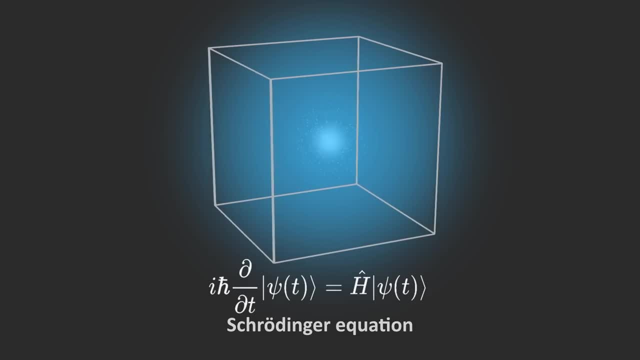 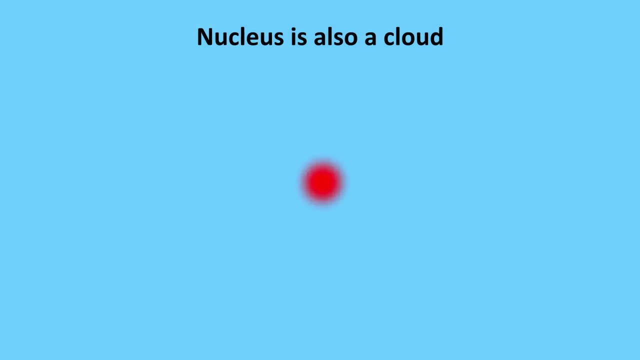 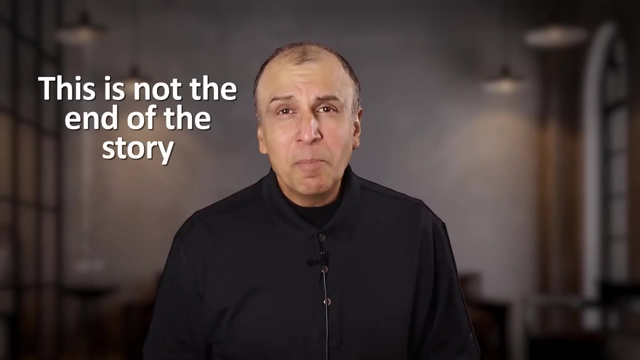 represents the probability cloud of the location of the electron. Note that the nucleus, too, would be fuzzy as well, since it is also a quantum object, but its cloud would be more localized than the electron's. You might think this is a great model. We know everything. now We can stop here, But 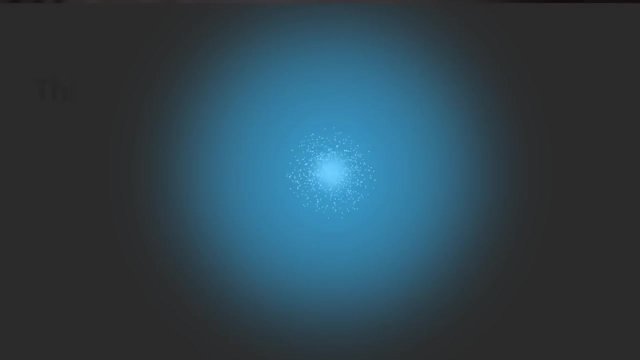 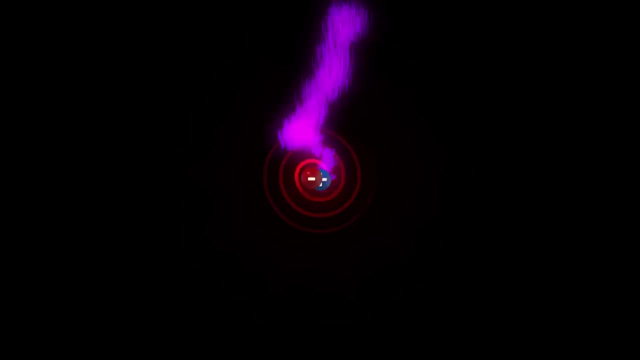 we can't, because quantum mechanics has some problems too. There are some things it can not explain, And we get the wrong results, Just like when we tried to explain the electron's orbit with the classical formulation. First of all, quantum mechanics is not relativistic. 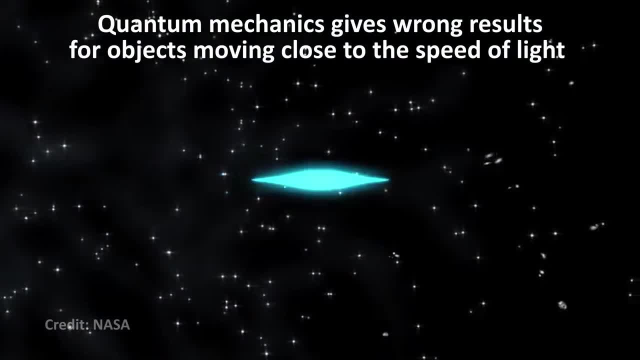 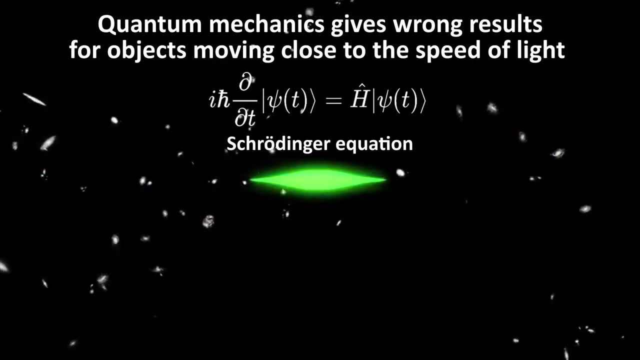 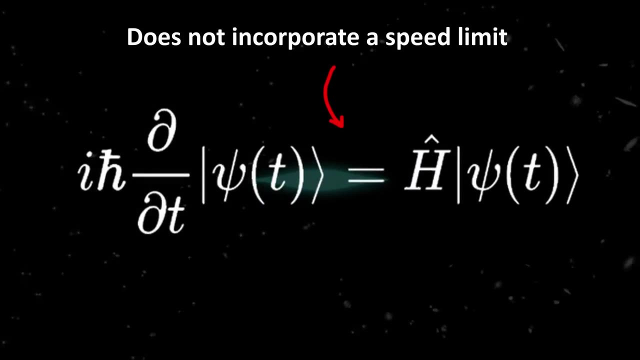 That is, it will give you wrong results. if the quantum object is moving close to the speed of light. Schrodinger's equation simply doesn't obey Einstein's theory of special relativity. The practical result of this is that it doesn't incorporate a speed limit – the speed of light – needed to make causality work, For. 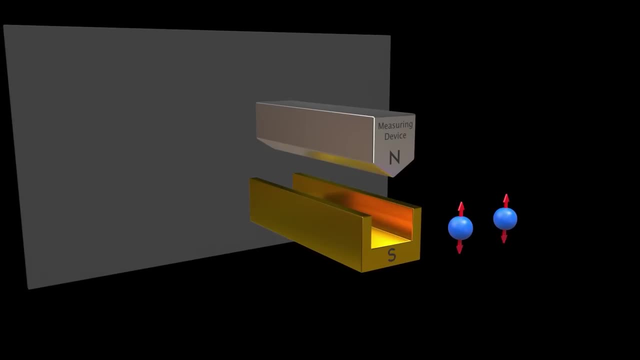 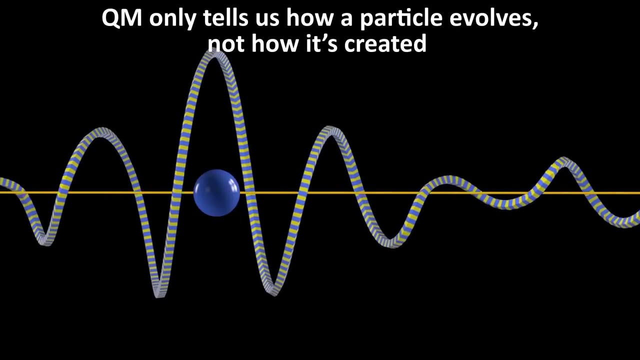 example, it allows for two measurements to influence each other faster than light. This would mean that there would be some reference frame in which the future could influence the past – breaking causality. A second problem with quantum mechanics is that it only tells you how a particle evolves over time – that is how it goes about its business. It does not tell you. 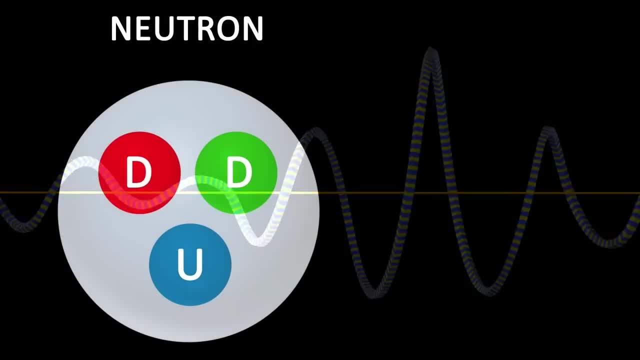 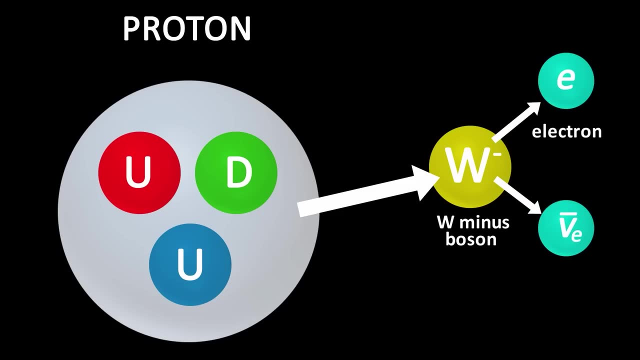 how it is created or annihilated, So it can't account for things like beta decay due to the weak nuclear force where a neutron transforms into a proton, an electron and an antineutrino- In this case quantum mechanics- breaks down. 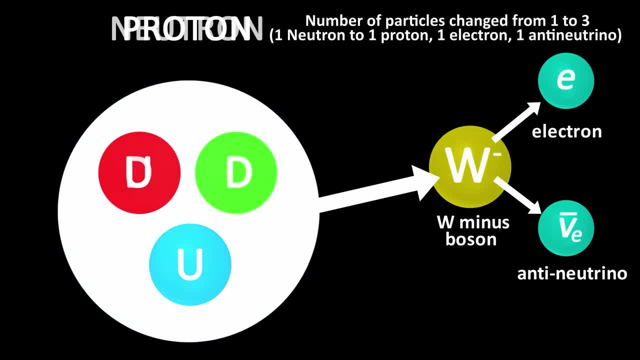 Because it doesn't work if we change the number of particles. In the case of the beta decay I just described, the down quark of a neutron decays into an up quark, changing the neutron to a proton, and at the same time emits an electron and an antineutrino. 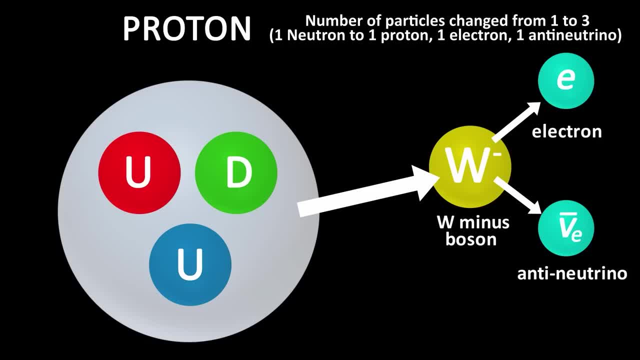 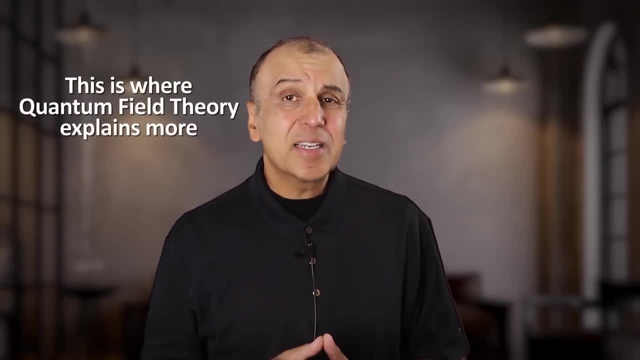 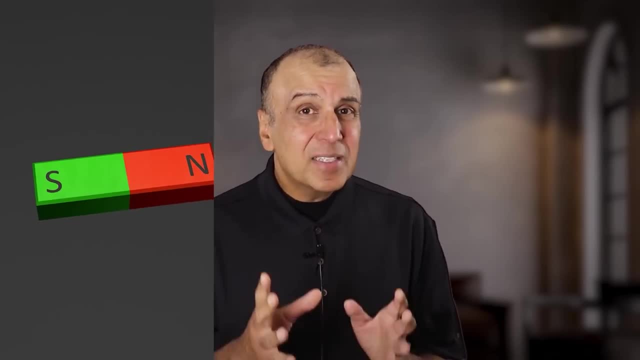 with a mediating W boson. This change to other particles can't be described by quantum mechanics. This is where quantum field theory explains things that quantum mechanics cannot explain on its own. So what is quantum field theory? Well, it's a mathematical framework that combines classical field theory – a classical field would 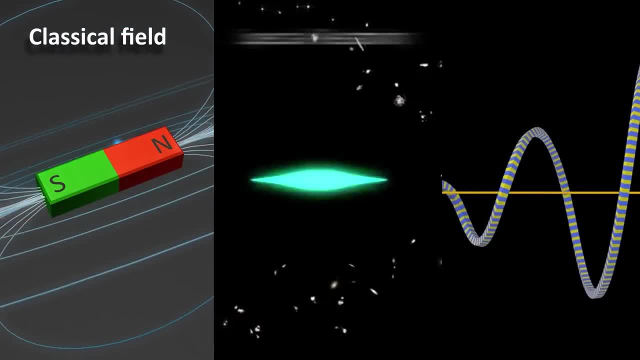 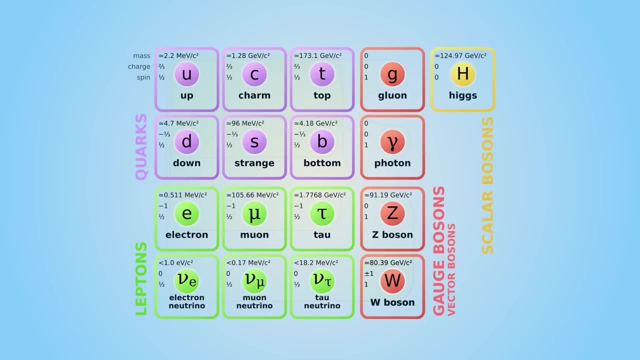 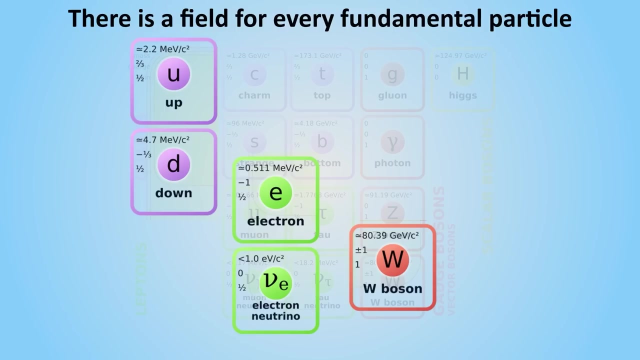 be like a magnetic field. as described by James Clark, Maxwell, special relativity and quantum mechanics, There is a field for every particle of the standard model. So in our beta decay example there would be a field for the down quark, the W boson, the up quark. 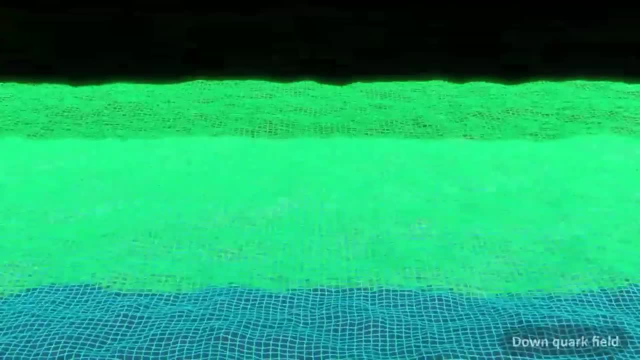 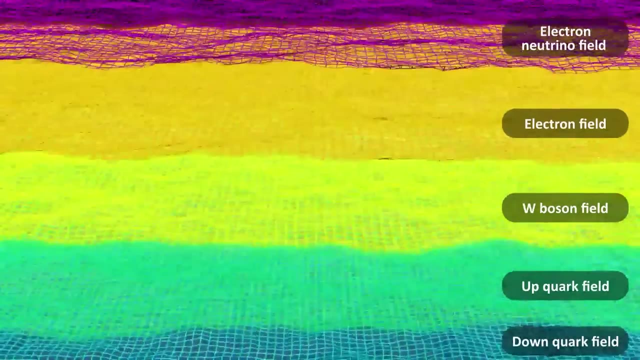 electron and the antineutrino. All these fields extend out in all of spacetime. In other words, the fields are always there and exist everywhere, including inside your body. Now, although they exist everywhere and you can't see them, they are not nothing. 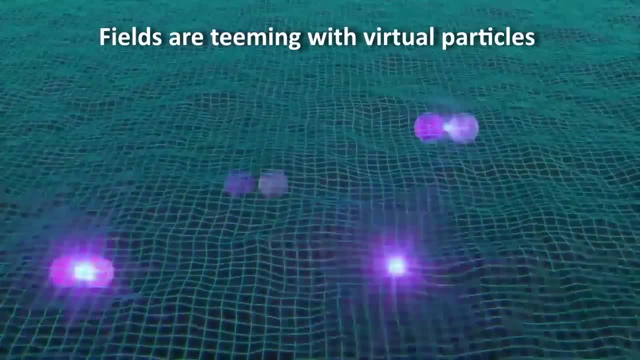 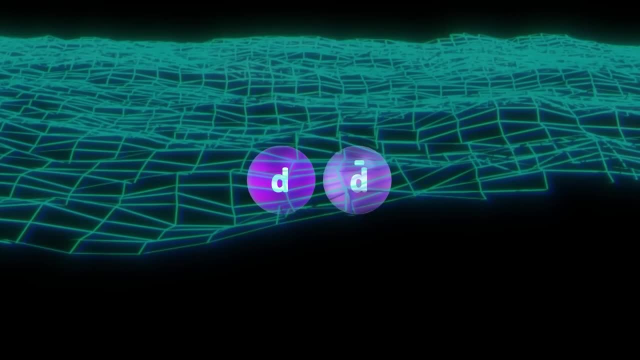 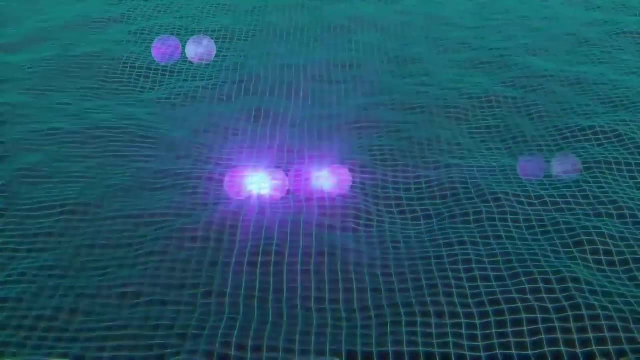 They are teeming with virtual particles. These are particle-antiparticle pairs that get created and destroyed. So, for example, the down quark field will always have some spontaneous creation of down quarks and anti-down quarks. They get created and annihilated almost instantly. They come in and out of existence constantly. 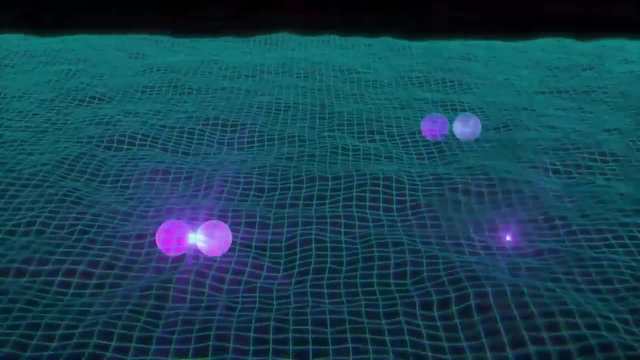 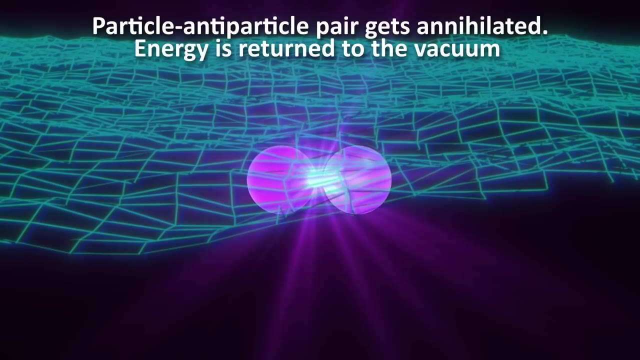 These virtual particles can't be measured. but nature allows the creation of these virtual particles by letting them borrow energy from the vacuum as long as that energy is put right back into the vacuum. This happens so quickly that it's as if nature doesn't register them as real. 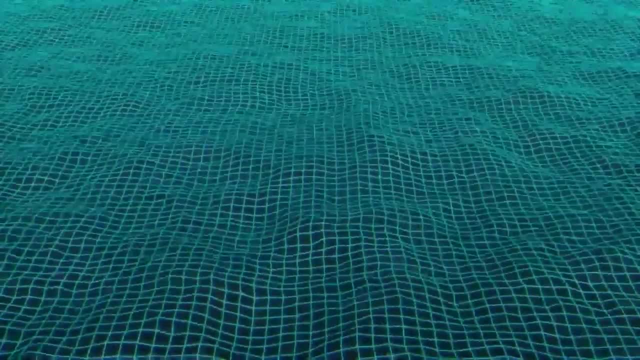 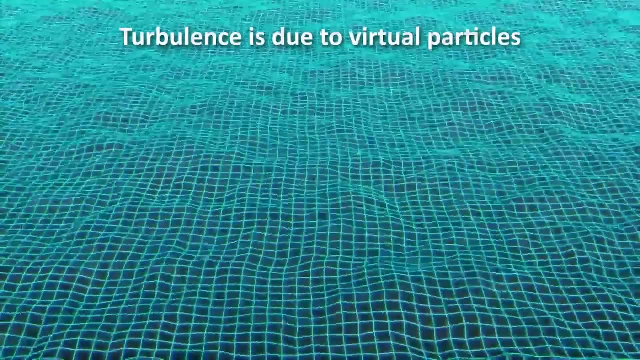 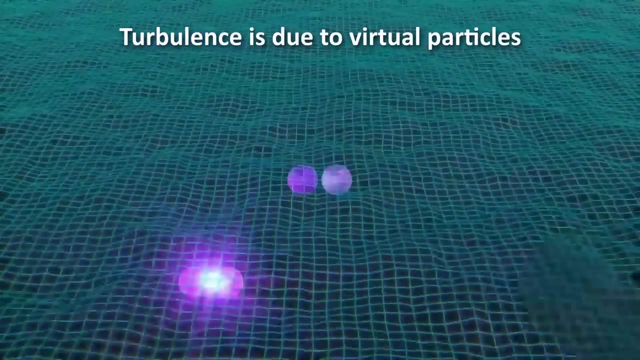 measurable particles. We can visualize these fields as a kind of ocean – just like the ocean wave has some turbulence, The fields always have a kind of turbulence, even in their ground state of minimal energy. This turbulence is due to the virtual particle creation and annihilation I just 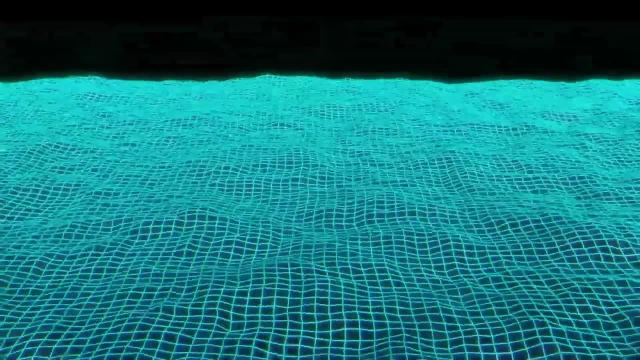 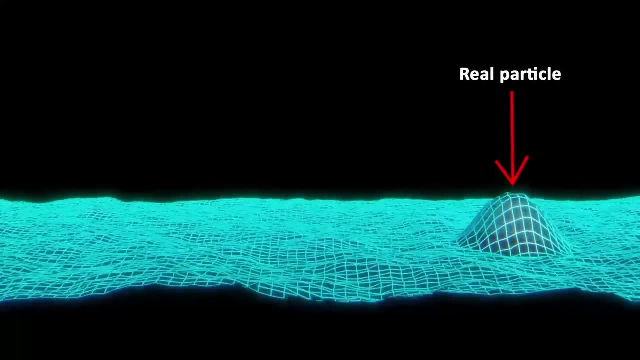 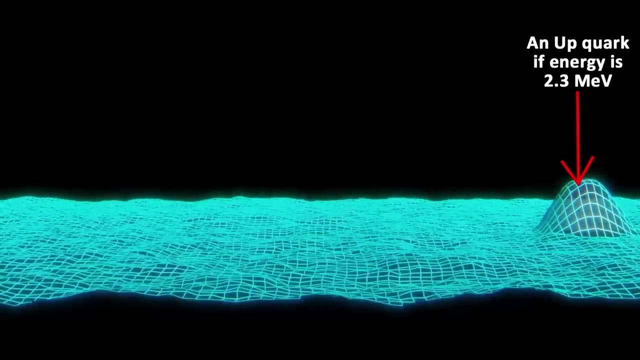 described. In these turbulent seas, if there is enough energy, a large wave can be created which can be measured. These are the real particles. So in the up quark field, for example, an up quark will be created if there is energy of 2.3 mega electron volts, or MeV, which is the mass. 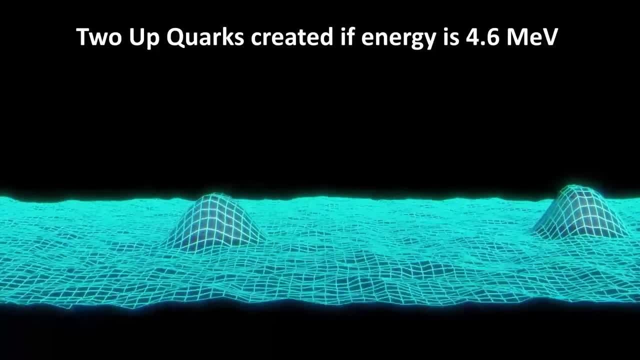 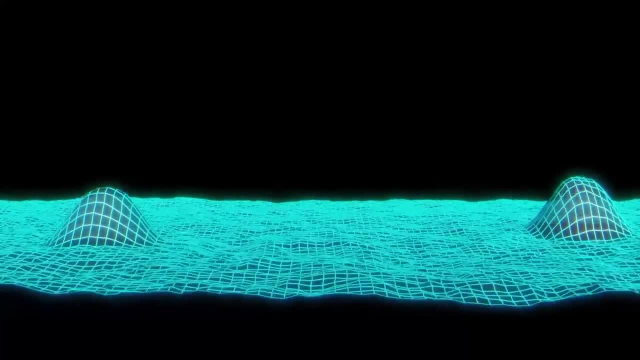 of a particle. Two quarks will be created if there is energy of 4.6 MeV. So a particle is nothing more than an excitation. in this field. These excitations are quantized, not continuous, So the fields can only create particles in integer increments. They cannot, for example, 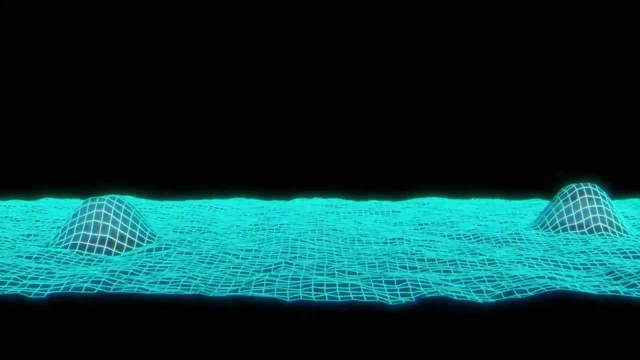 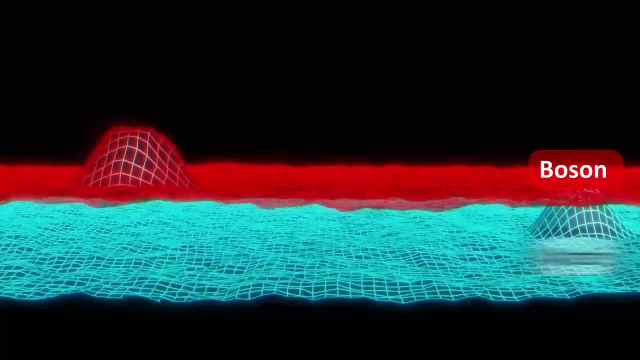 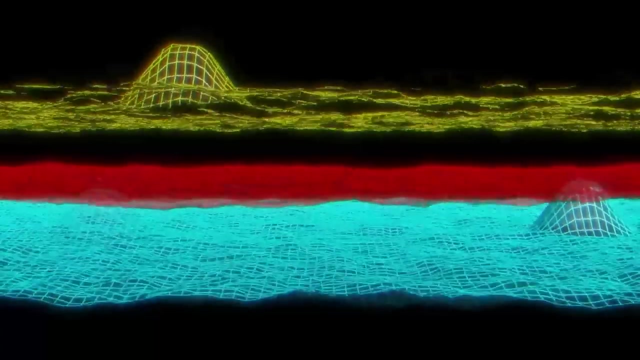 have one and a half up quarks, only two quarks or three quarks, etc. Now energy can be transferred between two fields via a mediating boson field. This is considered an interaction or a force. Particles can't interact on their own without a mediating boson. So while in quantum mechanics 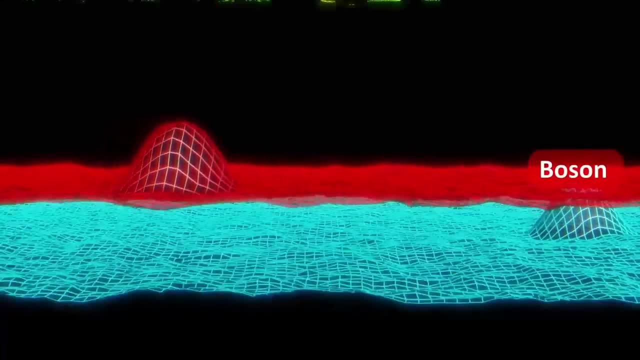 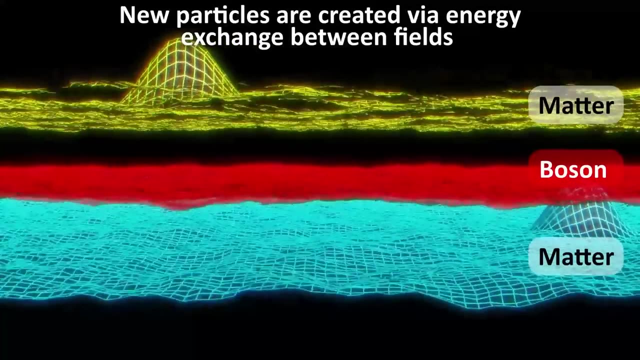 there is no way for the neutron to split its energy into three different particles – a proton, electron and an antineutrino – in quantum field theory, this can be done via energy exchange between the fields. You start with the fields of all the different particles, which are always. 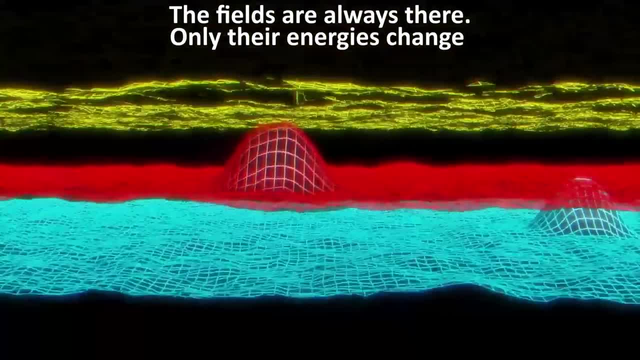 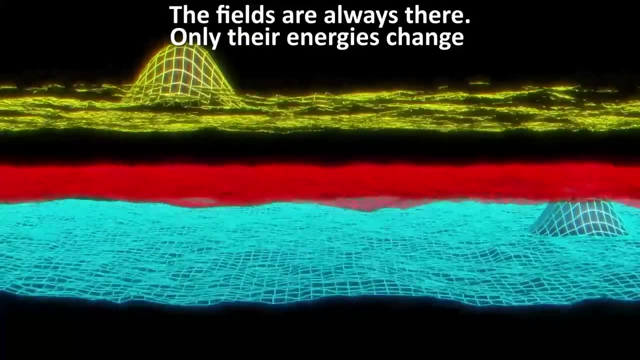 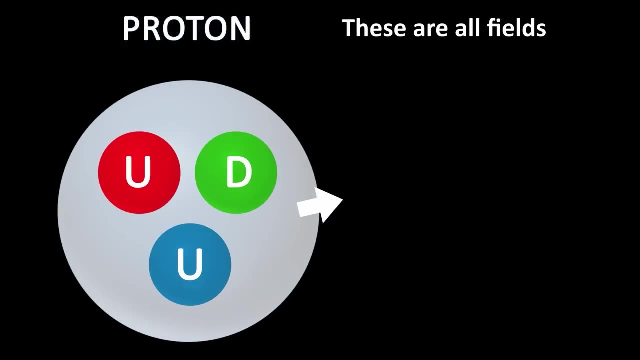 there and you finish with the fields of the same particles. Some of them just have more or less energy after the exchanges of energy. So in our beta decay, for example, we start with the down quark field. This field transfers its 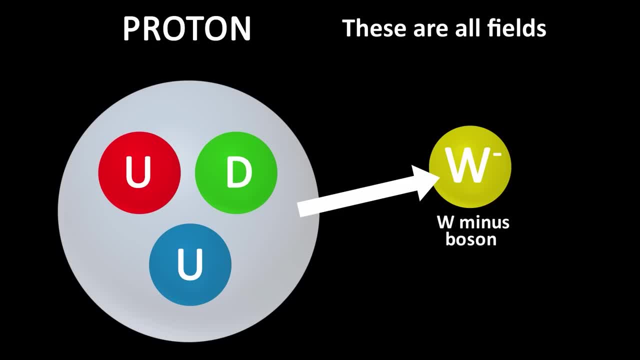 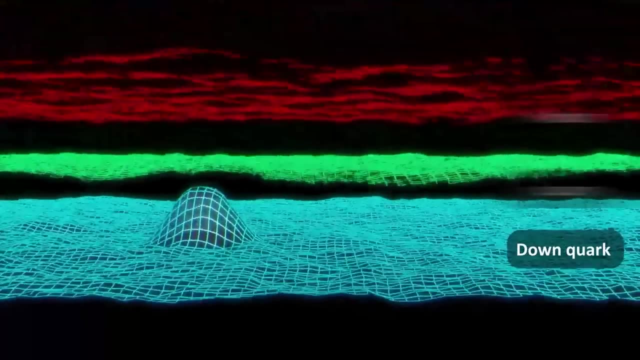 energy to the up quark field and the W boson field. The W boson field then transfers its energy almost immediately to the electron field and the antineutrino field. So we started with one particle in the down quark field and ended up with three particles simply by the fields. 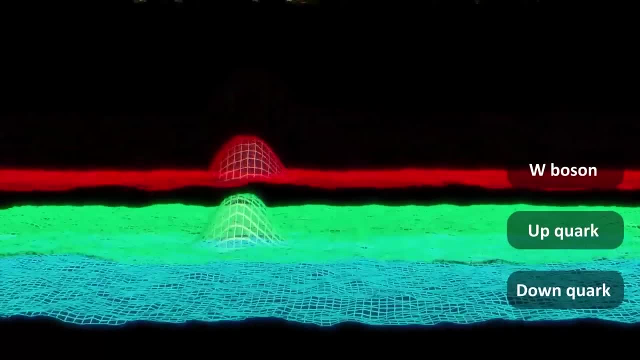 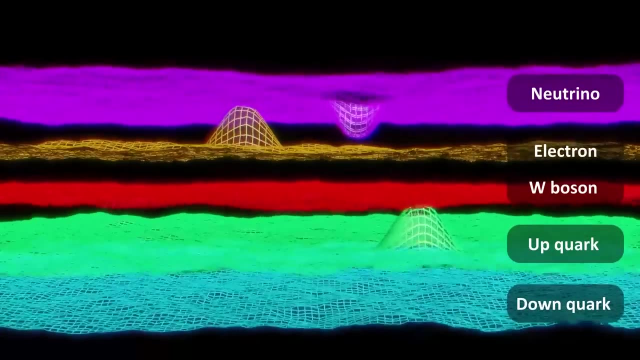 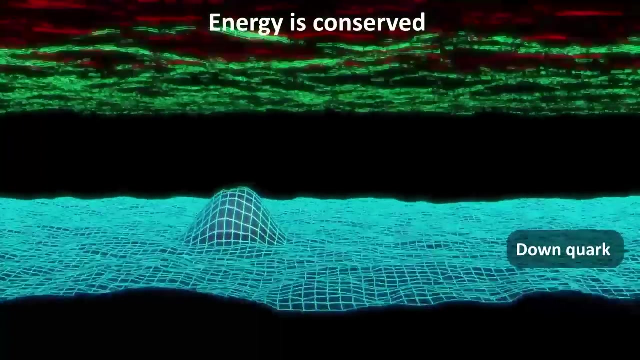 exchanging energy of particles changed, the total energy is always conserved. If you add up all the masses and kinetic energy at the beginning, they will add up to all the masses and kinetic energy at the end. In other words, the energy of the fields is the same before and after. 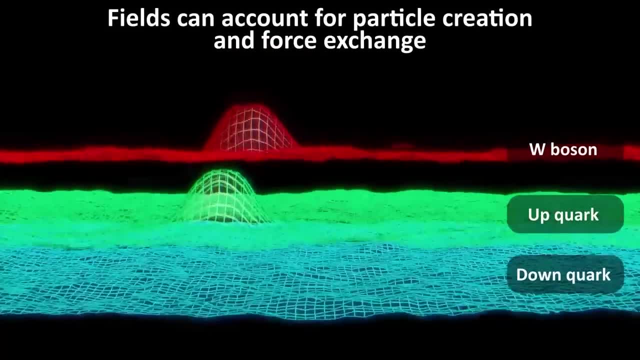 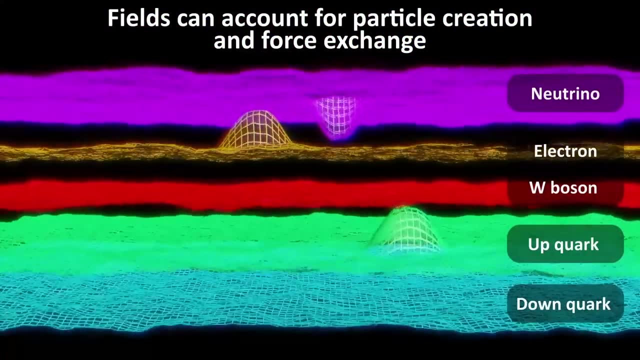 the energy exchange. So by having quantum fields we can mathematically account for and model creation-annihilation of particles, as well as the mechanism of force exchange. The icing on the cake is that the theory is fully relativistic, meaning it is free. 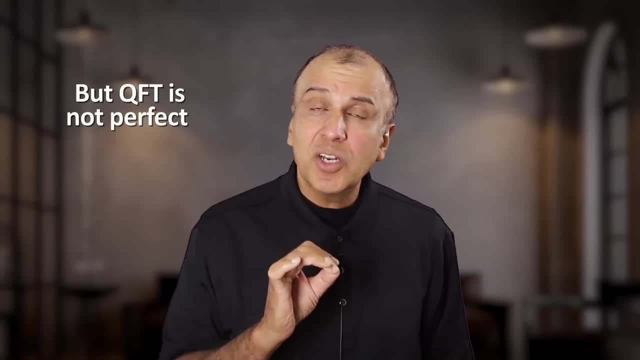 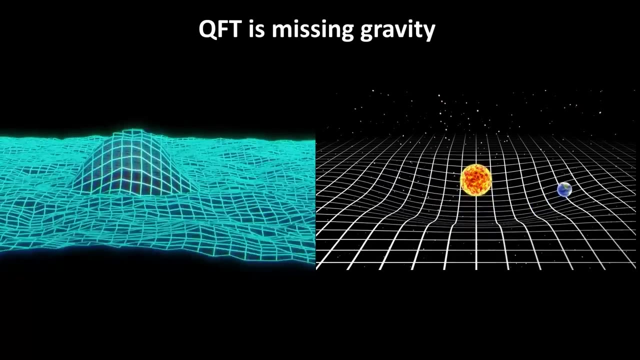 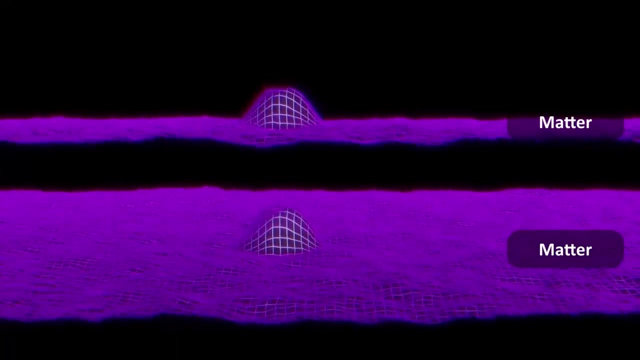 of causality violations. But even this modification of quantum mechanics is not perfect. For example, it's still missing gravity. We do not have a quantum field theory for gravity. If we did, it would mean that we could model a field for the theoretical graviton particles and gravity would be mediated. 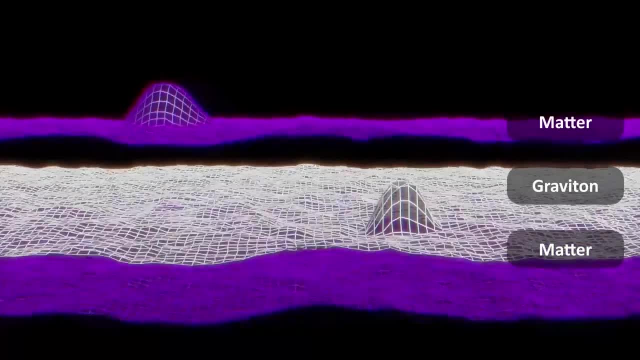 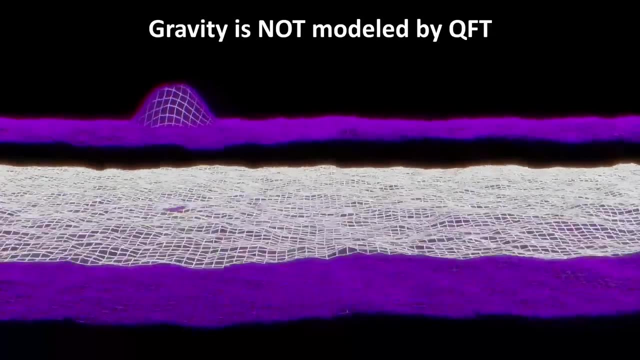 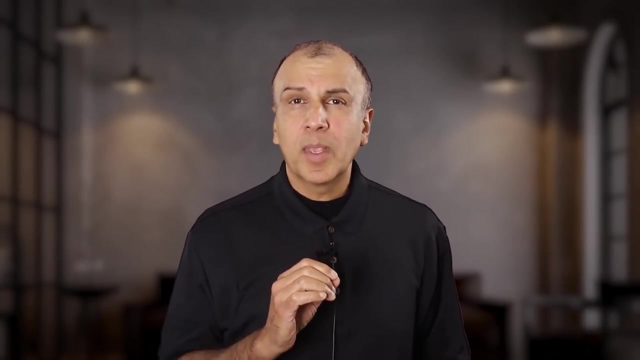 between matter particles by the exchange of this graviton boson. So even QFT, which is extremely accurate for the forces and particles we do know about in the standard model, remains as yet incomplete. The fact that we don't have this tells us something. It reminds me. of the saying that when you have a hammer as your tool, everything looks like a nail. Our tool is QFT. So far, everything we know has been a nail. So either gravity is not a nail or maybe we just don't really know how to use the hammer. 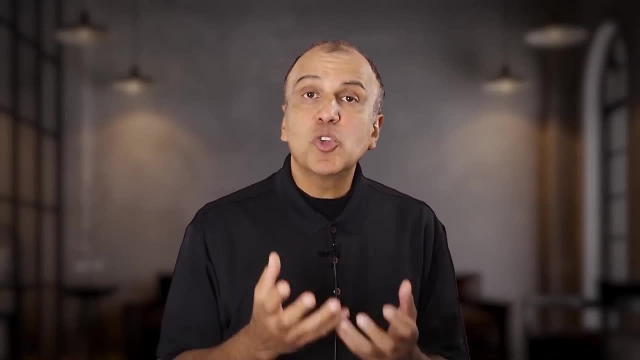 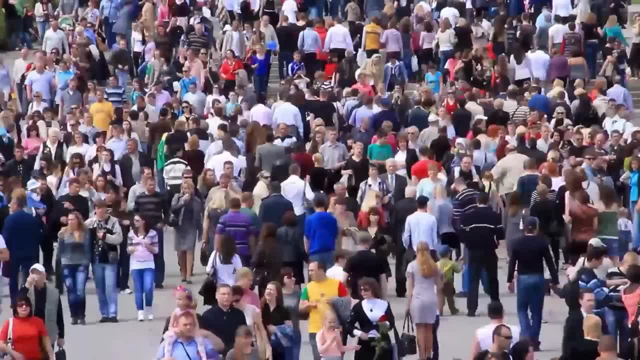 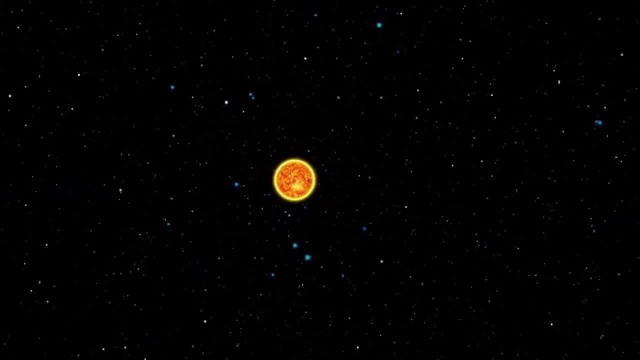 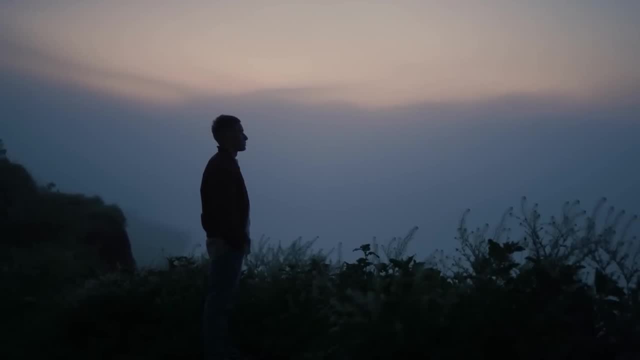 why? Because it tells us that the universe and everything in it, including us and all living things, the whole planet, every star, every galaxy and even things outside the visible universe, are all connected. Everything, even our thoughts, dreams and ideas, are 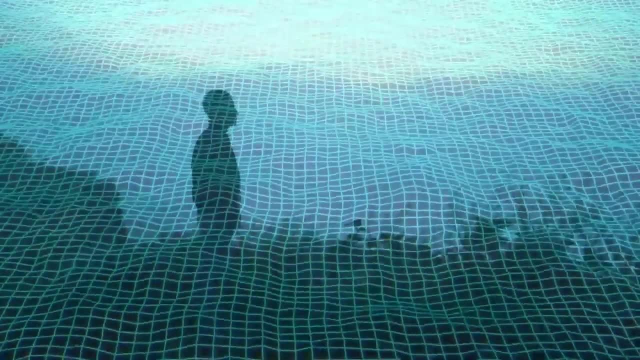 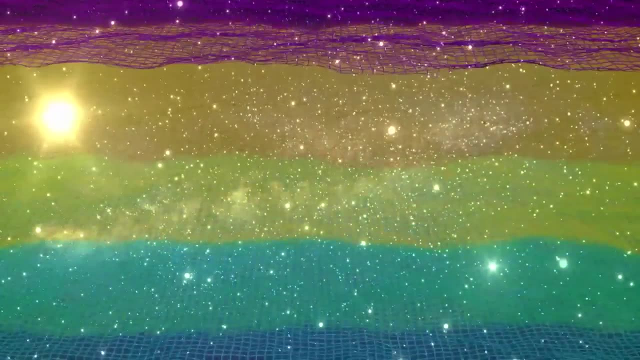 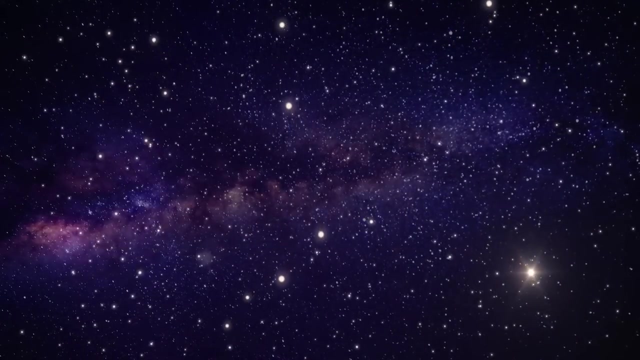 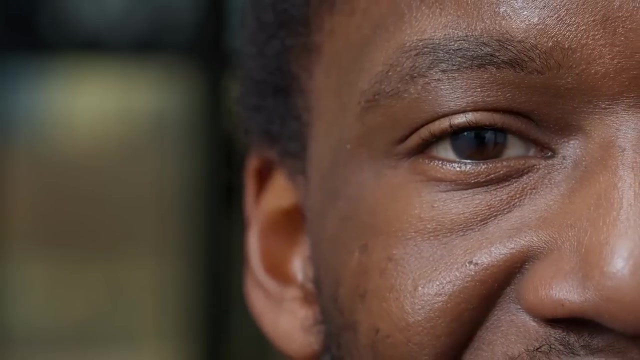 composed of excitations in the same quantum fields, And all these fields extend to the universe And we are all simply a series of excitations in it. So when someone says we're all one or that we are all connected to the universe, this is not just a fanciful idea. 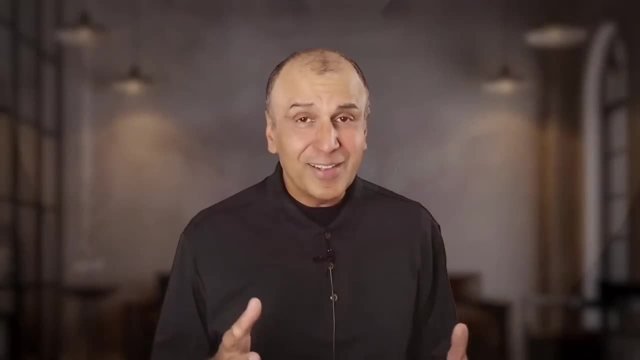 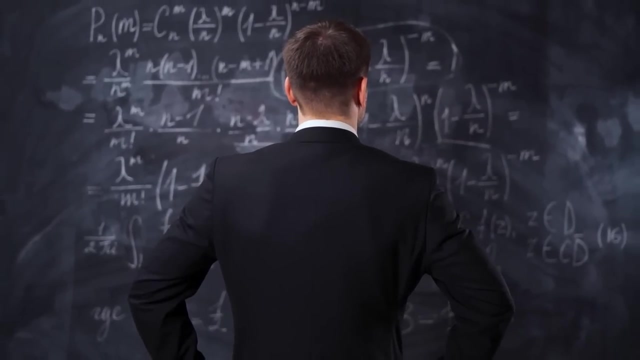 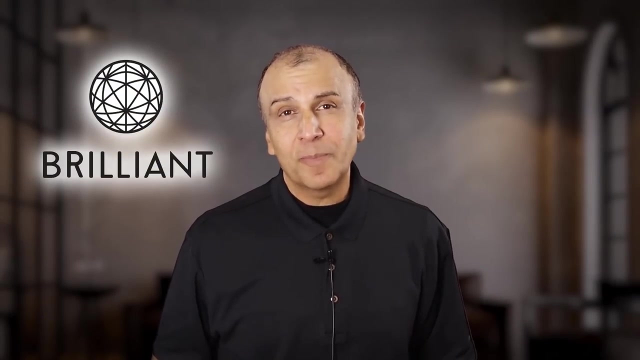 but has a real physical meaning. I find this to be beautiful. And another beautiful thing is that we humans happen to have the ability to actually comprehend the universe, at least to some degree, And Brilliant, our sponsor today makes that process simpler. One of their exceptional new courses is called Quantum.